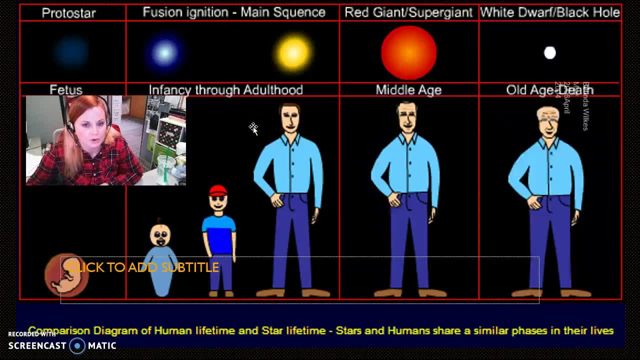 it's kind of like a baby who hasn't been born yet and during the time in which the star is growing like in the main part of its life, a time where it's growing and forming into a fully functional adult, and then it starts to age and that aging process isn't 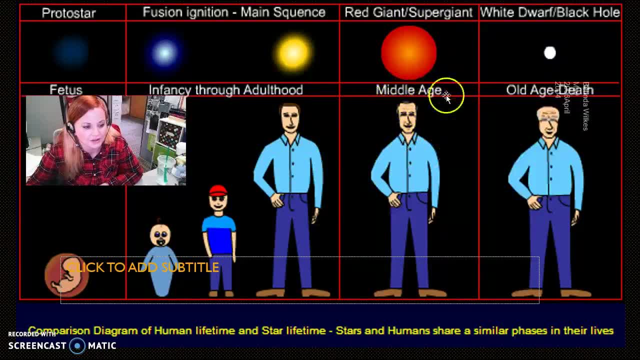 pretty It actually. you know. you see a lot of changes occurring, like you would when you are in middle age, like the red giant and super giant stars show, and finally, when you get to old age and death, you are a white dwarf and black dwarf star. So those are the 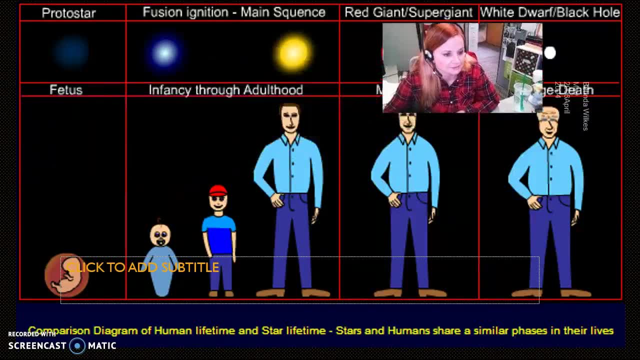 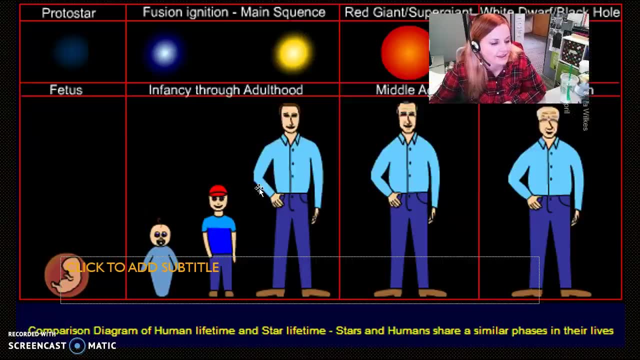 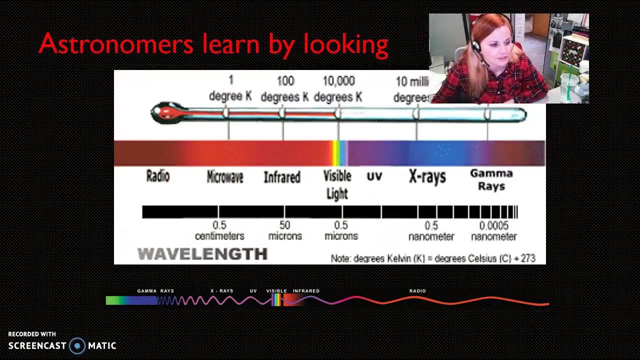 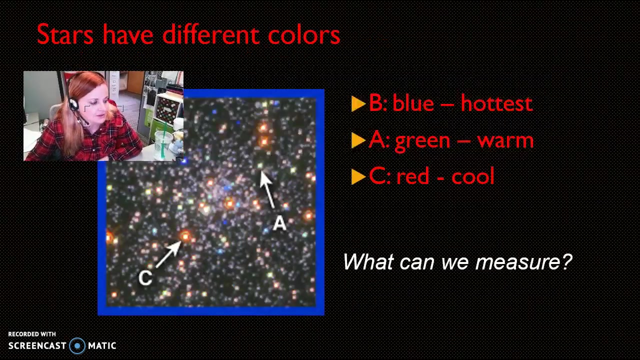 types of stages. So stars that we'll be talking about today are larger mass stars, and larger mass stars will appear blue to violet in color. They are higher temperature, just like we can see, this end of the spectrum is higher in temperature and therefore, and they're also higher in mass. 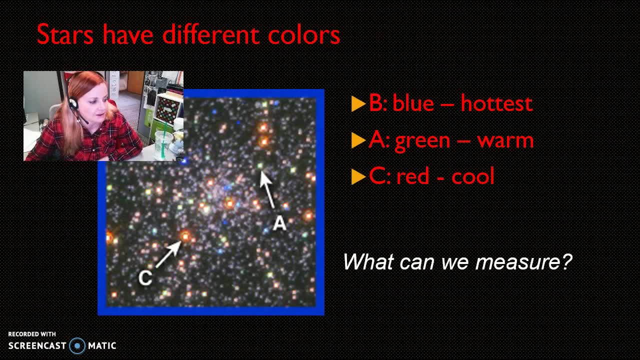 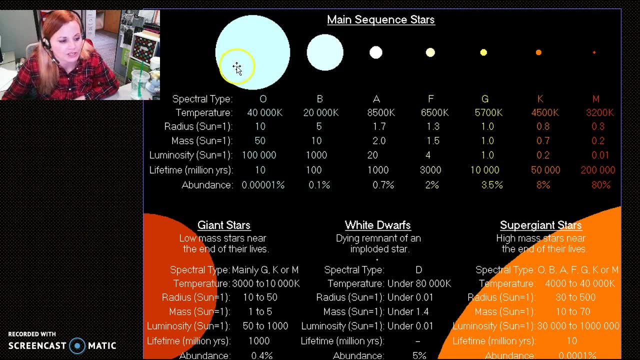 so they're bigger stars. Let's see if I can find a picture. It kind of illustrates to you the different sizes and temperatures of these stars. So these types of stars we're looking at are spectral types, OBA stars. They're going to have surface temperatures in the tens of thousands of degrees. 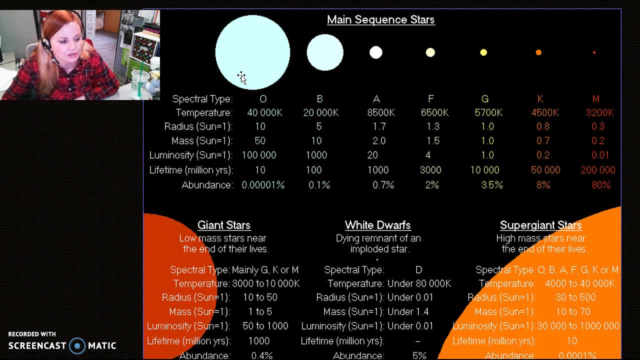 Kelvin, and they're going to have core temperatures that range to several hundred million degrees Kelvin for the temperature in the core. Now, this is due to the fact that these guys are just really, really big. Compare a spectral class G star, which is the sun, to a spectral class O star, and the difference in size is: 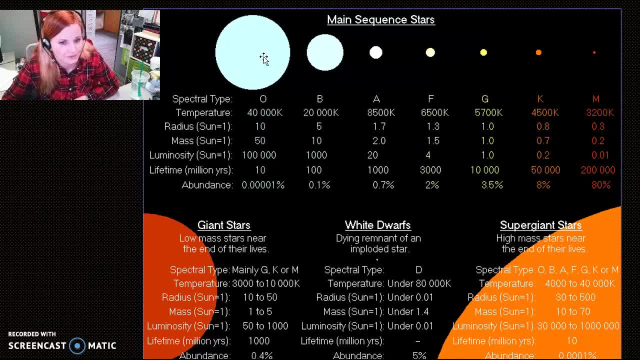 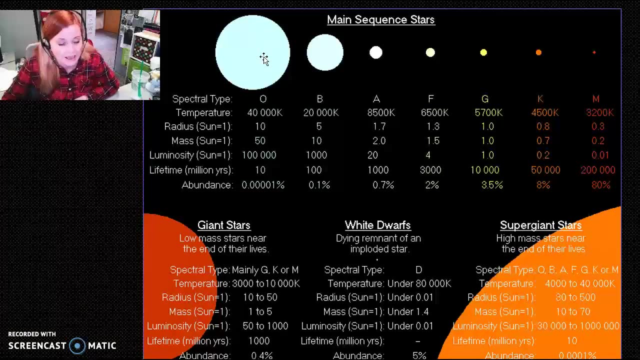 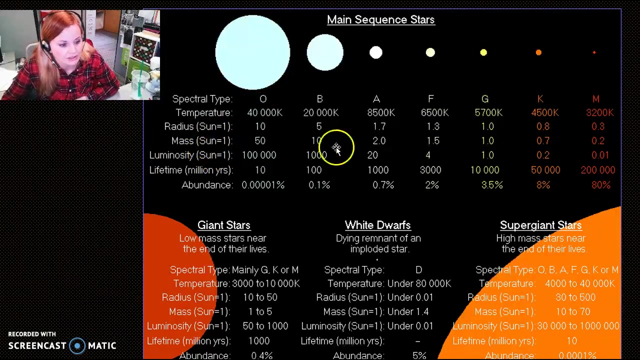 pretty astronomical. Hahaha, Pun intended, I guess, there. So basically, what's happening is that these guys they're burning really, really fast, That hydrogen is converting into helium at much faster pace, so even though they have more fuel, they go through it so quickly that their lives are very short compared to the Sun. 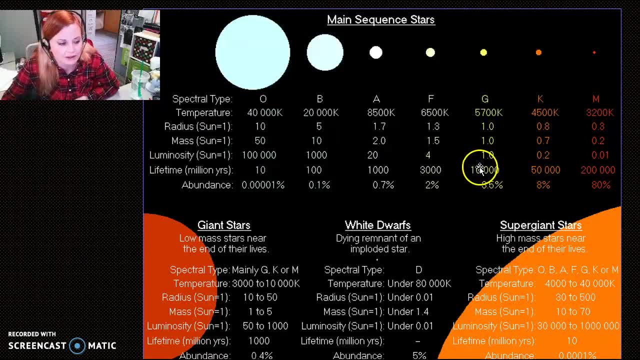 which has a lifespan of about 10 billion years. a big blue supergiant star is only about 10 million years, or a hundred million years for a somewhat smaller one right, and these are much more rare here because they are so large. the greatest majority of stars in the universe are actually these red dwarf stars, which 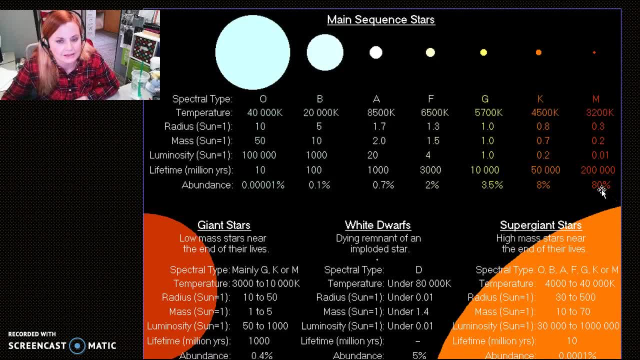 make up 80% of all stars. they're low mass, low temperature stars, low luminosity stars as well, and they have very, very long lifespans- upwards of, you know, 200 billion years, so longer than the actual age of the universe itself, when stars start to grow and change due to changes inside of them, when they 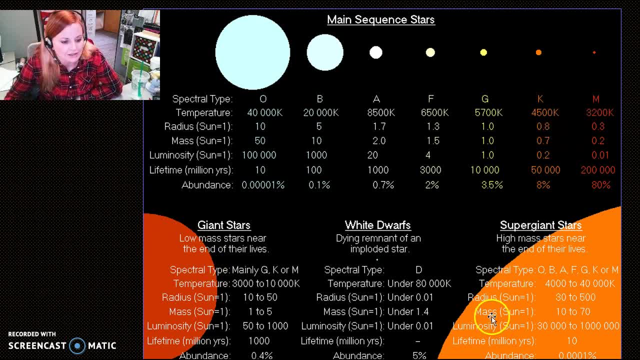 start to grow old, they change into these stars, giant stars and supergiant stars, and you can kind of see there again, the difference in size is pretty. it's pretty astronomical, right. so that's the differences we're talking about, and and let's look at exactly why this is. 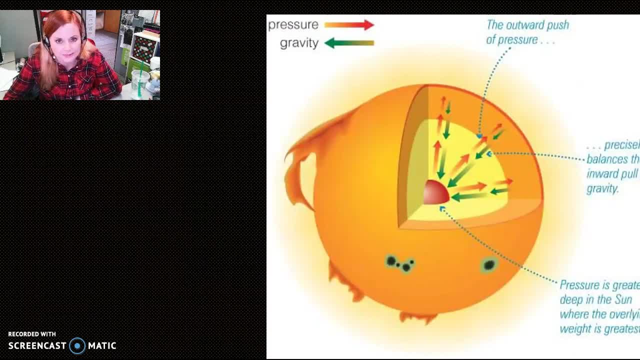 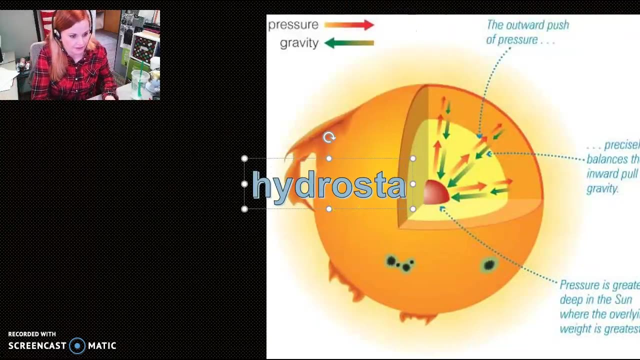 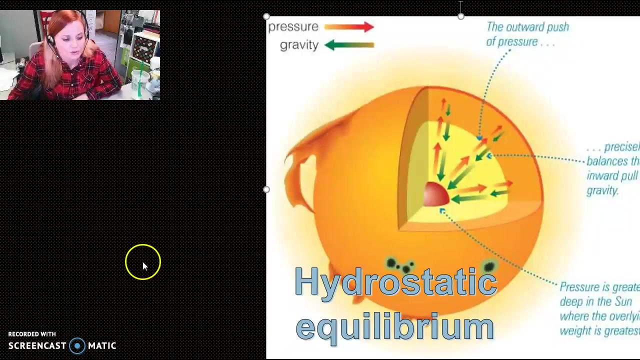 occurring, and I did talk to you about this in previous podcasts as well, but there's a special type of state that a star is in and it is called hydrostatic equilibrium, and I'm gonna- I'm gonna type that here for you guys. so hydrostatic equilibrium, basically, is referring to a state where the external 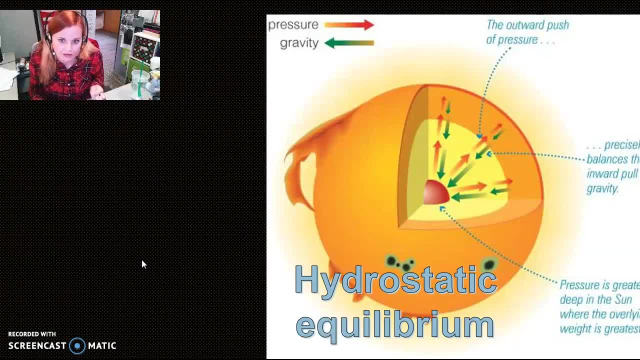 pressure pushing, you know, pulling that star together, that's gravity. pulls that star together is equal to the outward force that comes from those nuclear reactions in the core. so the hydrogen converting into helium is an explosive force and this is occurring. you know an exponential level, but it's equaling the 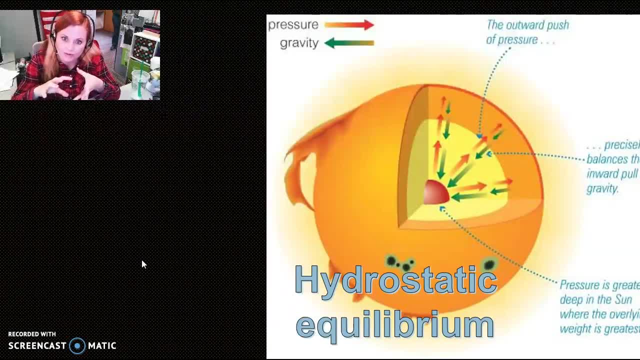 force of gravity, so the star remains very stable and doesn't change in the future. It's giving off heat and light and all sorts of different types of electromagnetic radiation. the other thing that's occurring is, you know, you have this core that's made up of hydrogen, and that hydrogen is fueling into helium after a while, though. all of that 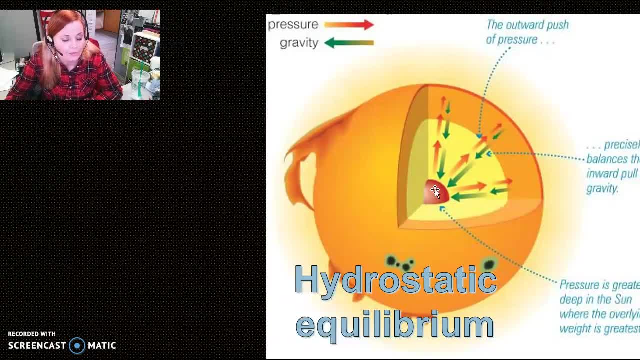 hydrogen in the core becomes used up, and when this happens, that's when we start to see changes. if you take away the arrows pushing outwards and you only have those gravitational arrows pulling in, The star is going to shrink, and when it shrinks, it collapses. it gets much, much hotter and 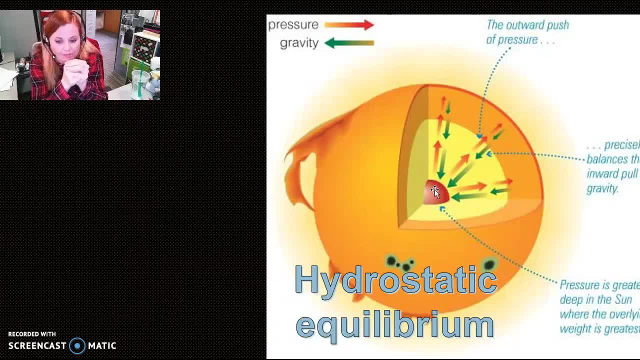 it becomes much more more dense, lots of pressure and heat. it becomes so much more pressure and heat that helium can now be forced together to fuse hydrogen. so that's occurring, so that is going to cause those outward arrows coming back again. So the star will then expand and in addition to that there is another layer of the star. 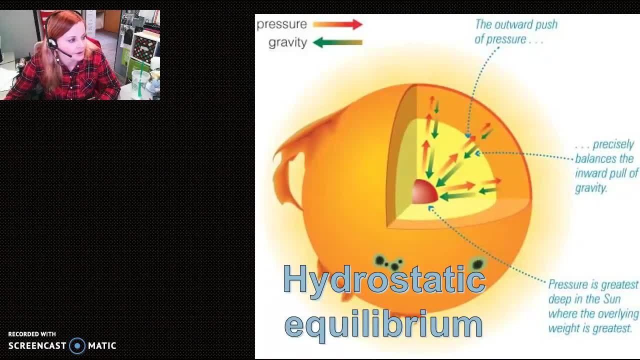 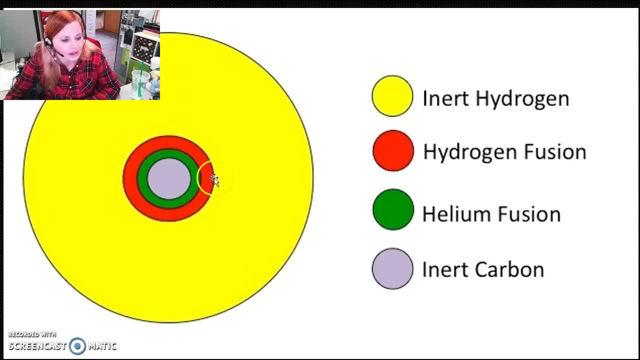 If you go back to this one. no, so what actually happens with these high mass stars is that you'll have helium fusing, fusing into carbon in the inner part of the core, but then you'll have another ring where hydrogen is still fusing into helium. so so that's happening. 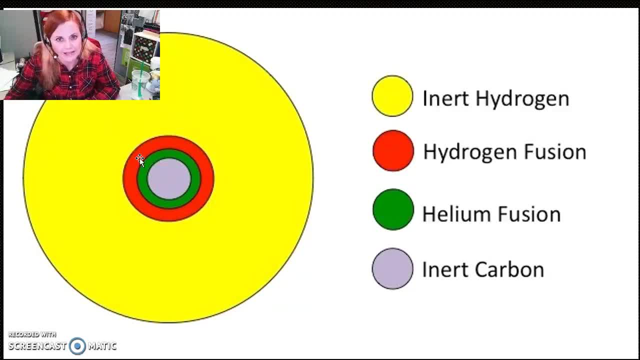 as well. So There are two levels of fusion going on in these high mass stars. so that's increasing those outward forcing arrows. so now it gets even bigger than it was before and that's why you have these stars developing into red supergiants rather than just red giants. they 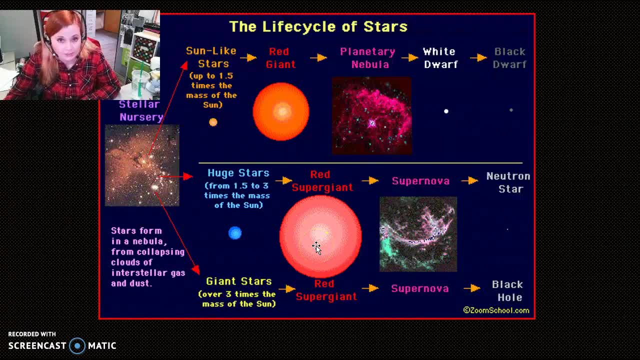 become these big, red supergiant stars. now this process goes on and on. after a while it's going to run out of helium and then it will shrink again because, again, no outward arrows. So you can see the liquid that's trying to force families. 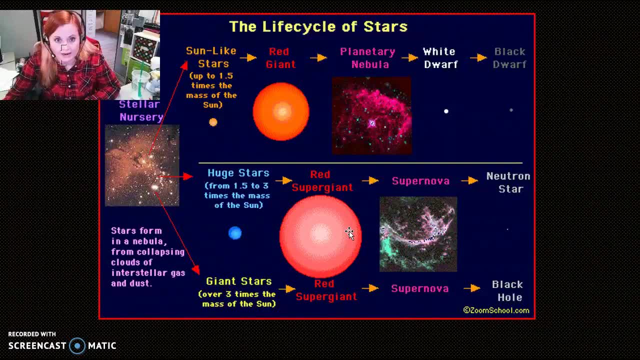 And you know something's happening with this thing. So let's go back to that point of oxygen плат year. so the number of puts that There's an element. That's why you can imagine the amount of oxygen and that's why there's so many more. 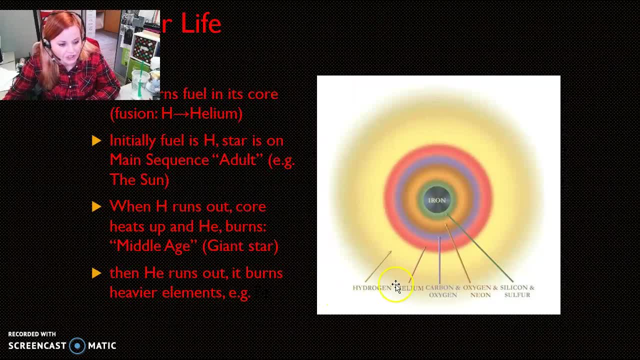 put-put團veis. Lets talk about stronger screening. So if you're trying to process something, is that the oxygene isn't in carbon. there's starch, titanium that's gone into nitrogen, so up into the oxygen point of oxygen isn't the limit limit and then that really is Somewhere there's more Lower layer of oxygen and then 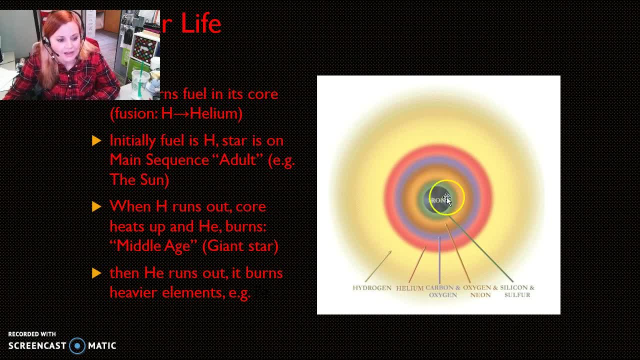 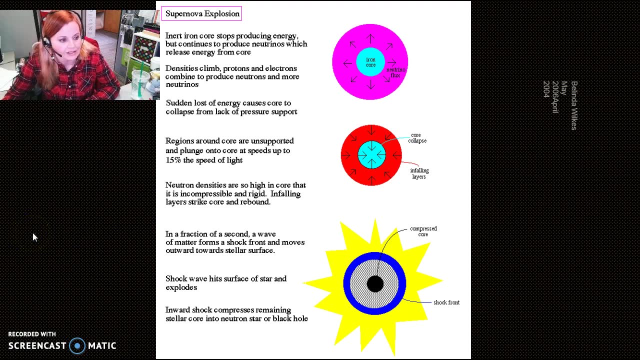 the same time. What eventually happens is you end up with a core that is made of iron, And this is a very, very dense core. In fact, it's so dense that the iron core produces neutrinos which are releasing from the core. These are basically just neutrons that are moving, And protons and 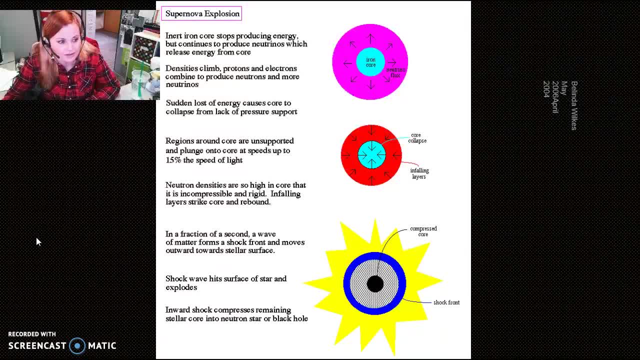 electrons combine to make more neutrons and neutrinos, And then we have the star collapsing again due to the loss of fusion. But because the core is so dense, this time you don't get the compression that you had before. Instead, you get this rebound effect and it collapses and 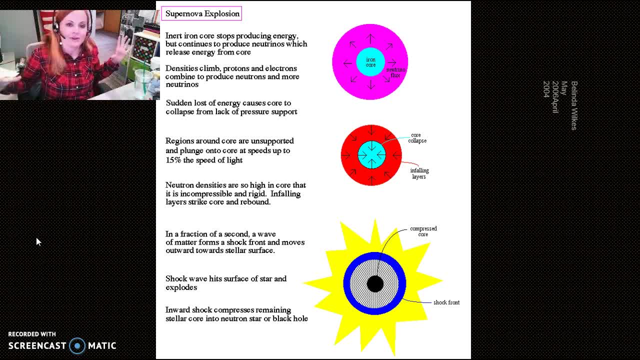 basically rebounds off that iron core and bursts outward in a supernova explosion. right, So that's what a supernova is, It says. in a fraction of a second, a wave of matter forms a shock front that moves outward towards the stellar surface. The shock wave hits the surface of the 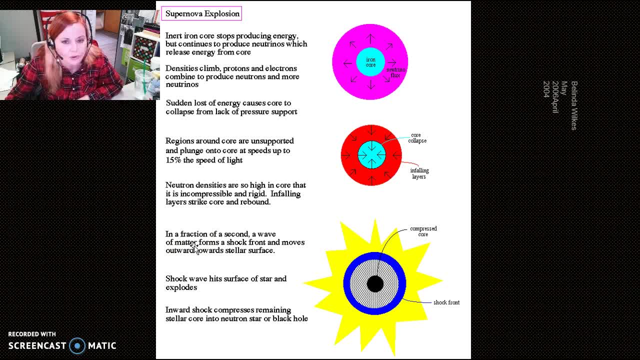 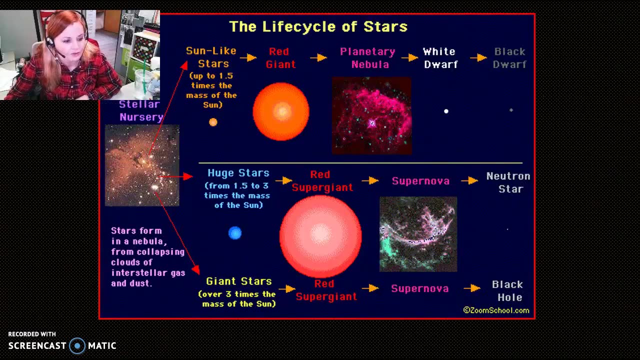 star and explodes, The inward shock compresses remaining stellar core into a neutron star or a black hole. So then we need to ask ourselves, you know well, what does it become- A neutron star or a black hole, and why? Well, a neutron star is going to form from a 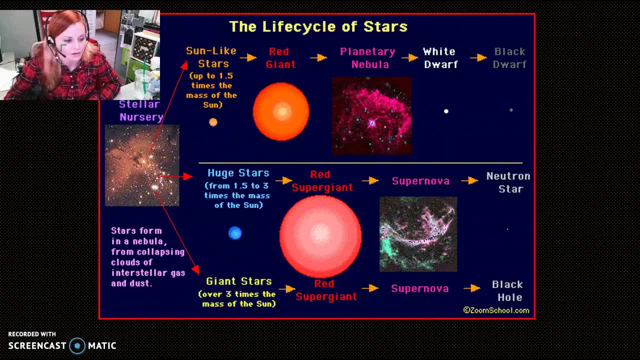 bigger neutron star. A neutron star is going to form from a bigger neutron star And that's going to form from a bigger neutron star And that's going to form from a bigger neutron star And that's star, something that's about, you know, one and a half to three solar masses. so 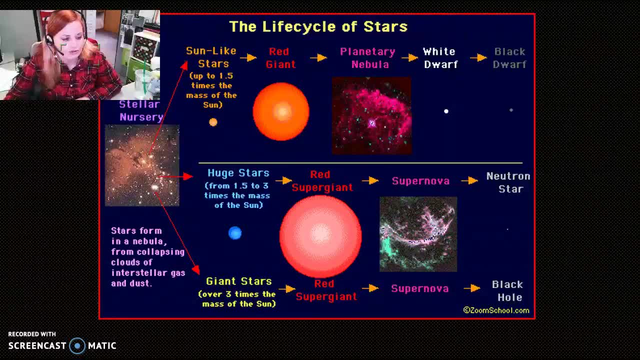 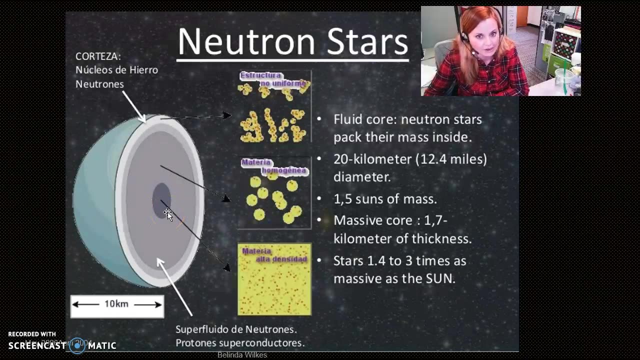 bigger than the Sun, but not super huge. anything that's greater than three solar masses will form a black hole. so let's talk about the difference between a neutron star in a black hole. so what we have here is one potential ending of a kind of medium sized, high mass star, and that is something called a neutron star. 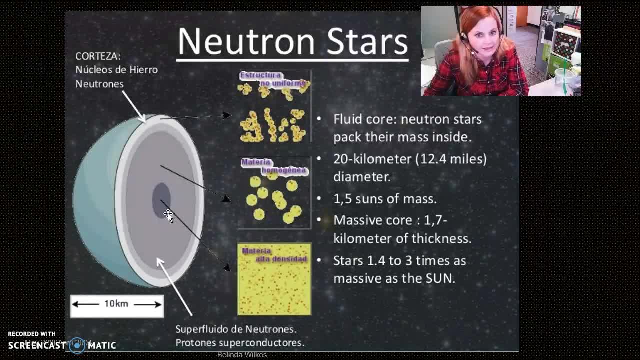 now a neutron star occurs when that last amount of fusion is done in the core and the core or the star collapses under its own gravity. you do have the first rebound in that supernova explosion, right, but what's left over is that you have the neutrons of the atoms, but you also have the protons that have combined. 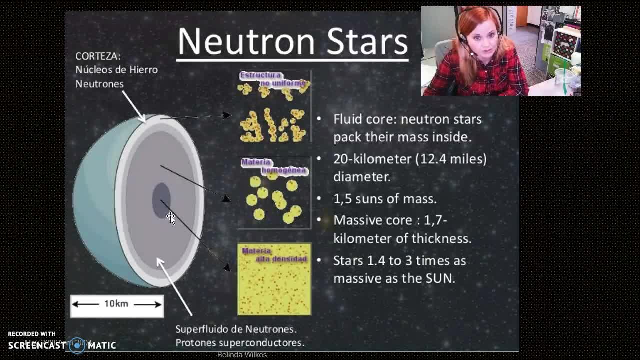 with the electrons to produce neutrons, then they also produce neutrinos as well. these are some particles that are streaming away from the neutron star. now what happens as it collapses is it begins to spin faster than it was before. it's already rotating, just like all stars are. 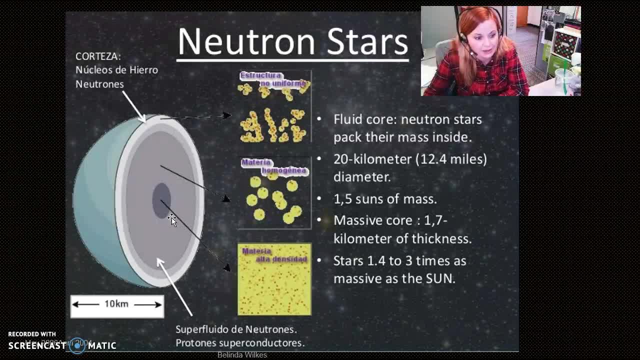 rotating, but it spins faster and faster, and faster the smaller it gets. neutron stars can be between 20 and 10 kilometers wide, so not very big at all compared to an actual large mass star right, but they are as massive as a one and a half suns right. so they're really really massive for their size just. 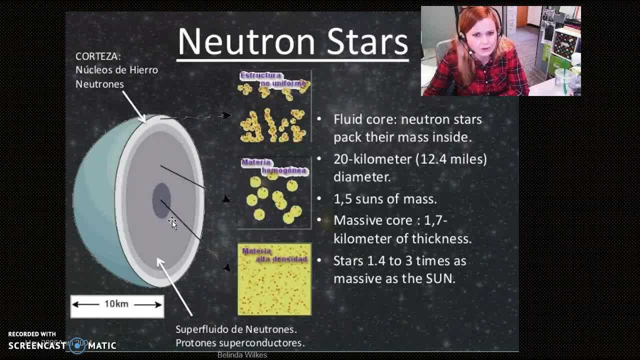 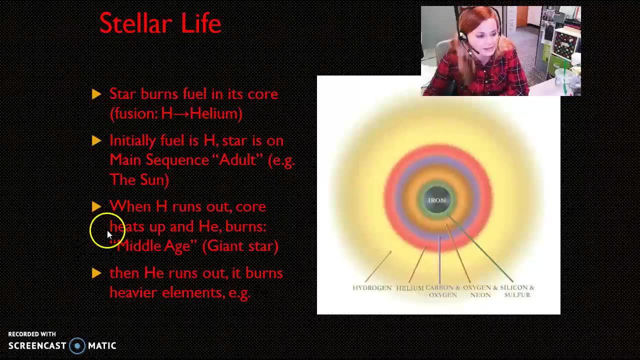 exceptionally massive. a teaspoon of a neutron star would weigh a hundred million tons, to give you kind of a analogy there. so these are for your medium high mass stars. for the higher mass stars, ones that are greater than three solar masses, you end up with a black hole. now, black holes are not. 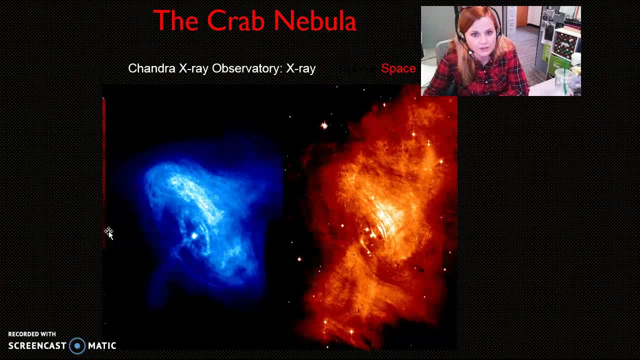 directly observable. they aren't something you can see, because what happens in a black hole is that the gravity is so strong that, in order to go fast enough to escape the gravity, you would have to travel faster than the speed of light, which is impossible to do so. not even light can escape a black 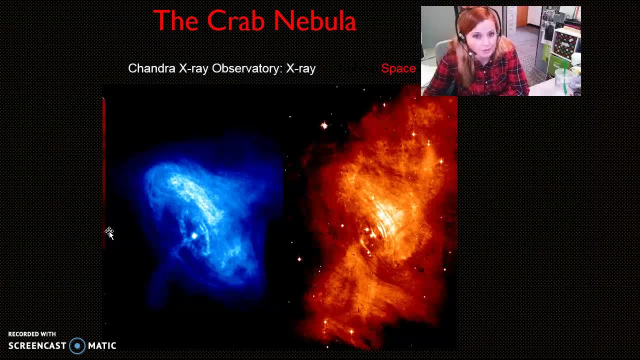 hole. that's why it's called a black hole, because nothing can escape a black hole. they can't directly be measured, but they do sometimes swallow neighboring stars if the star is close enough and in its gravitational field, and when that happens, oftentimes high frequency radiation is given off in the form of x-ray radiation, and so we have special 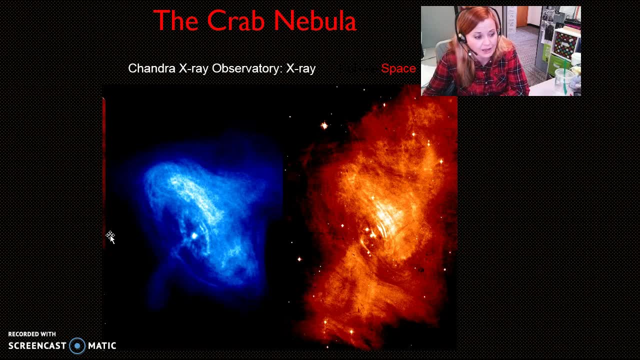 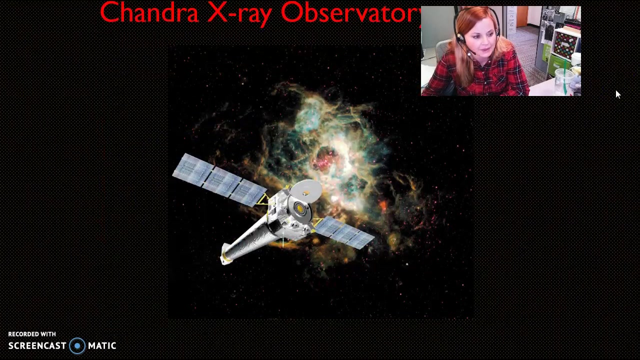 special telescopes, that is, are equipped to observe an x-ray radiation. thus the Chandra x-ray observatory does this and can take pictures of this energy, as it is kind of just just kind of being pulled into that event horizon of the black hole. okay, so that is kind of the end of this part of the the life cycle.